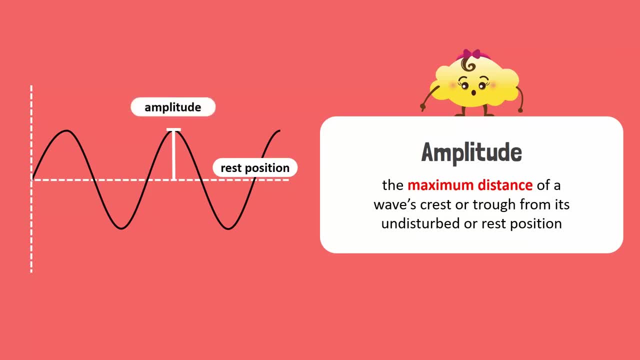 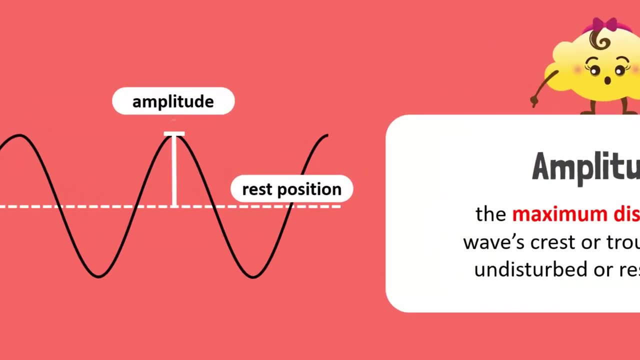 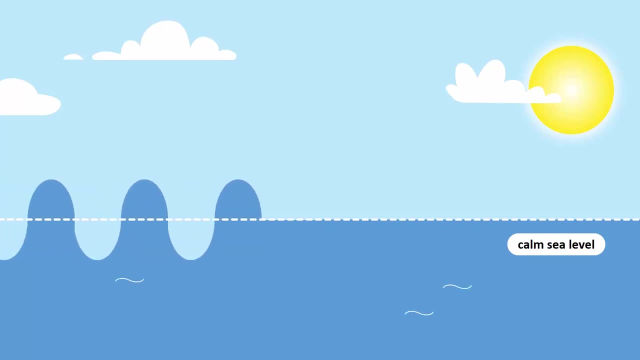 The amplitude of a wave is the maximum distance of a wave's crest or a trough from its undisturbed or rest position. Think of a calm sea and then an incoming wave. The amplitude is the height of the top of the wave from the flat sea level. 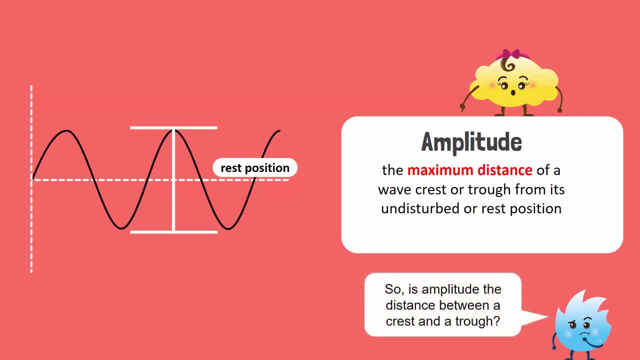 So is amplitude the distance between a crest and a trough? No, It is the distance of either the crest to the rest position or the trough to the rest position. Therefore, the vertical distance between a crest and a trough is in fact equal to two amplitudes. 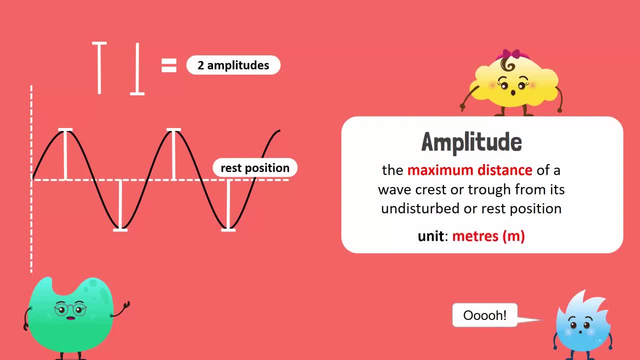 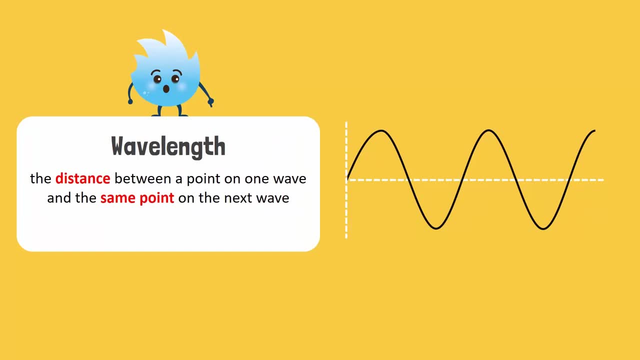 Oh, The amplitude of a wave is measured in meter m. Next let us discuss wavelength. A wavelength is the distance between a point on one wave and the same point on the next wave. For example, these two points can either be two consecutive crests or two consecutive troughs in. 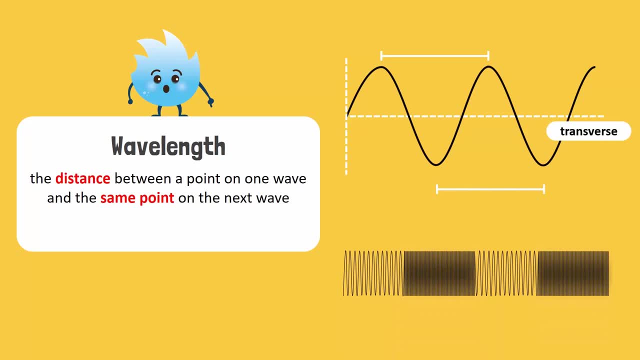 transverse waves, or they can be the distance between two consecutive compressions or rarefactions. in longitudinal waves. The wavelength is also the length of one complete wave. It is denoted by the Greek letter lambda and is usually measured in meters m. 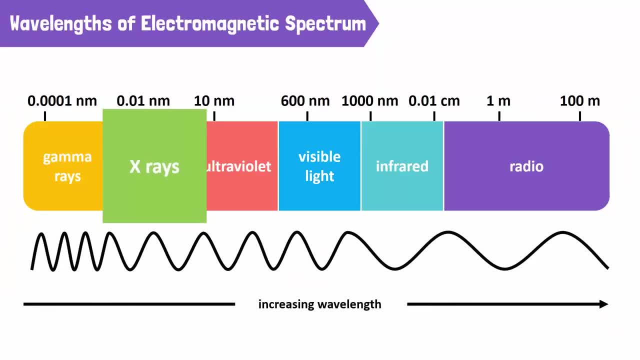 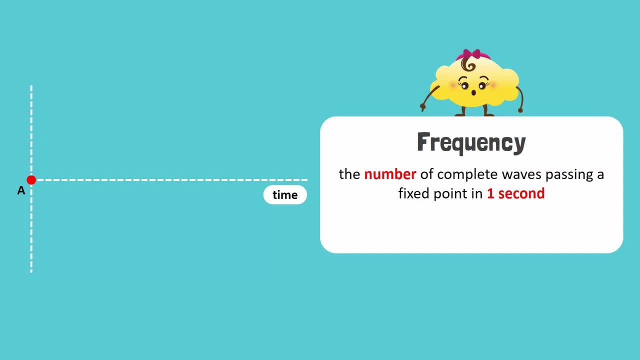 The wavelength can vary greatly. X-rays are very short, visible light is somewhat long and radio waves are much longer. The frequency of a wave is the number of complete waves passing a fixed point in one second. Frequency is given the symbol f and is measured in units called. 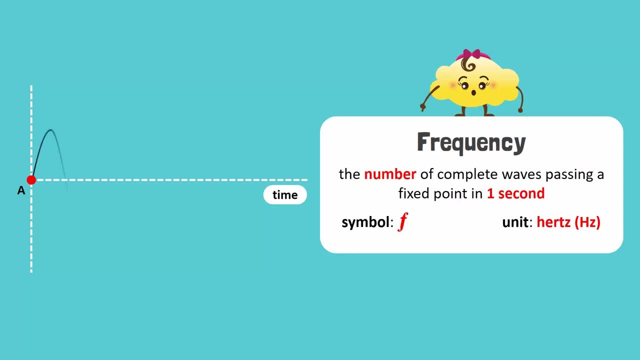 hertz. Let's look at this wave which is travelling from left to right. Can you count how many waves pass through point A in one second? Observe that in one second, exactly three waves pass through point A. Therefore, the frequency of this wave is three hertz. 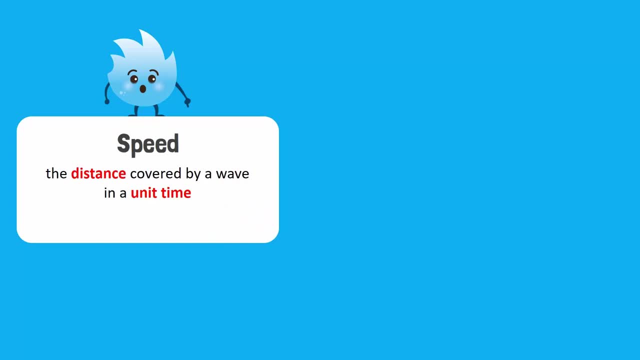 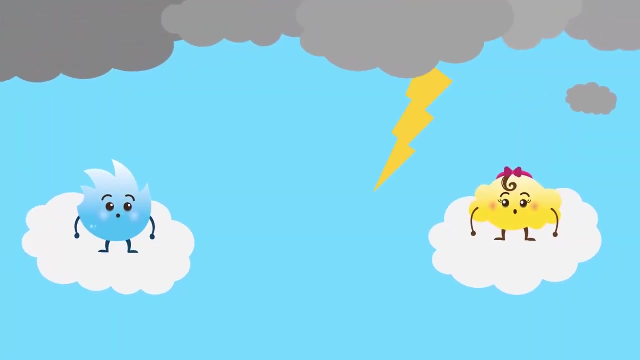 Lastly, let's discuss speed. The distance covered by a wave in a unit time is called its speed. Speed is measured in meter per second. Imagine seeing a flash of lightning and hearing the thunder of clouds. First we will see the flash of lightning and a few seconds later we will hear thunder. 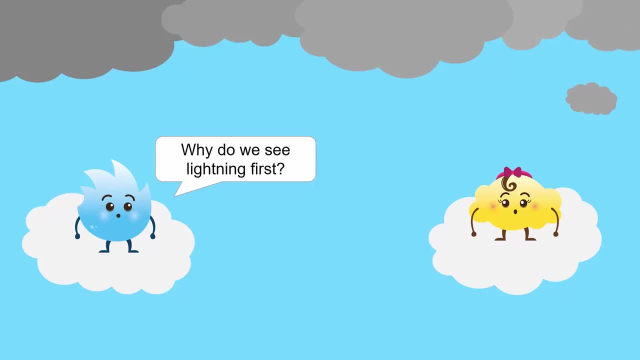 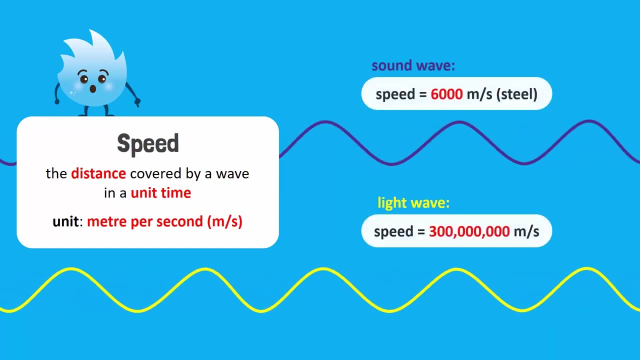 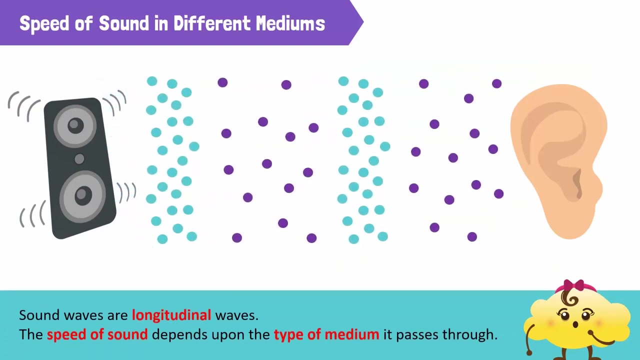 But why do we see lightning first? This happens because both light and sound are waves that travel at different speeds. Light waves travel faster than sound waves, So we see the light before we hear the sound. Sound waves are longitudinal waves, But the speed of the sound depends upon the type of the 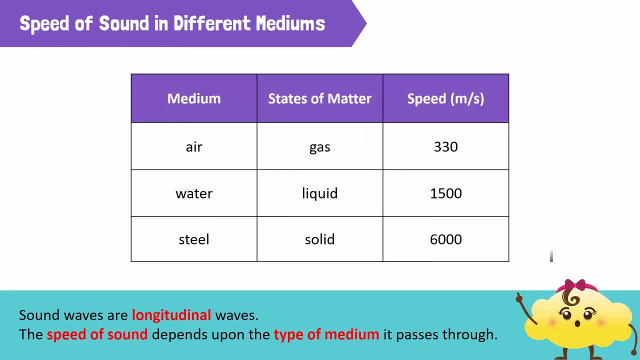 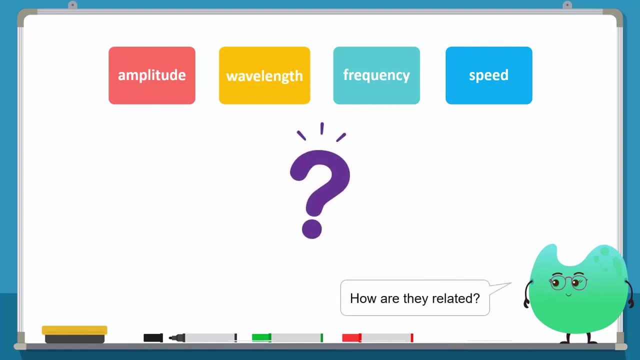 medium it passes through. Look at this table: Sound travels fastest in solids, then in liquids and the slowest in air. Now that we have seen the four quantities, how are they related? Well, it turns out that the speed of waves is the product of the wavelength and the frequency. 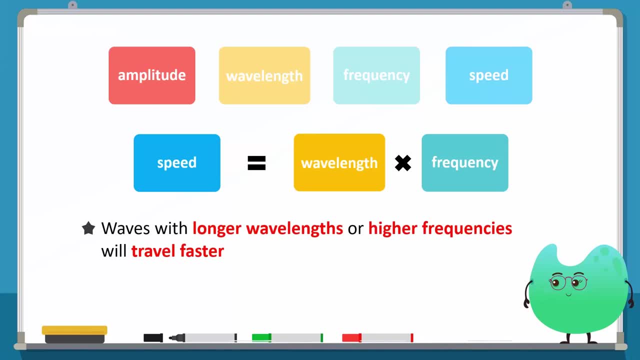 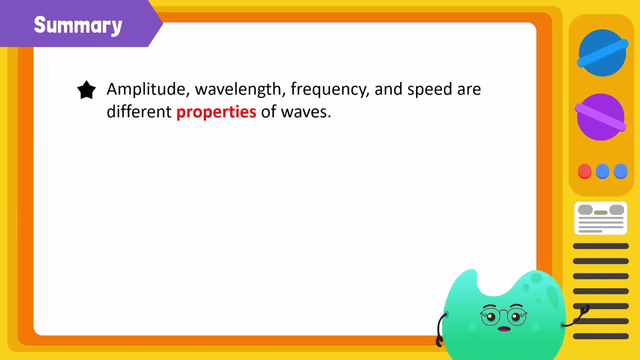 Therefore, waves with longer wavelengths or higher frequencies will travel faster does not depend on its amplitude. Today we've learned that amplitude, wavelength, frequency and speed are different properties of waves. Amplitude is the maximum distance of a wave, crest or trough from its rest position. 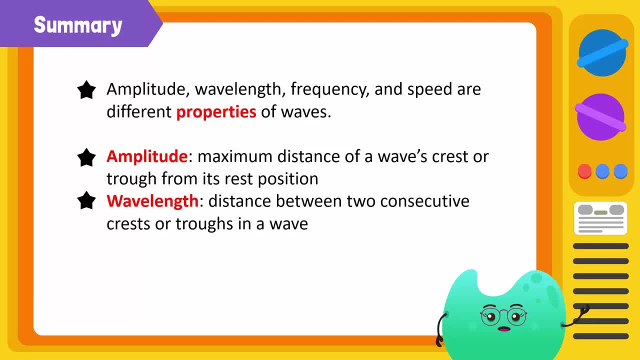 Wavelength is the distance between two consecutive crests or troughs in a wave. Frequency is the number of waves that pass through a fixed point within one second. The speed of a wave is equal to the product of its wavelength and frequency.